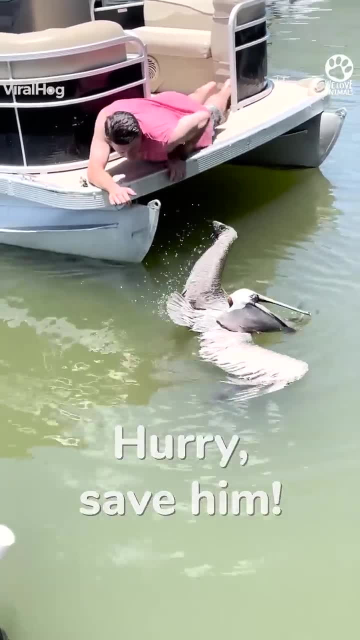 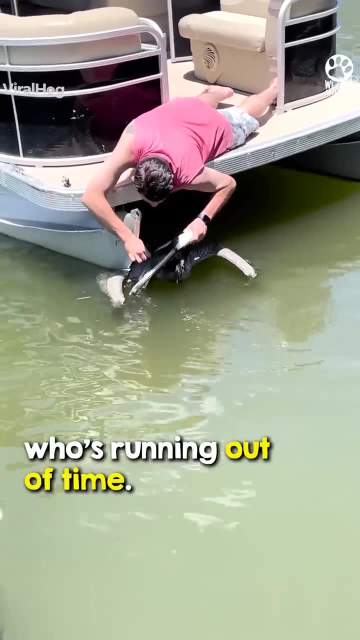 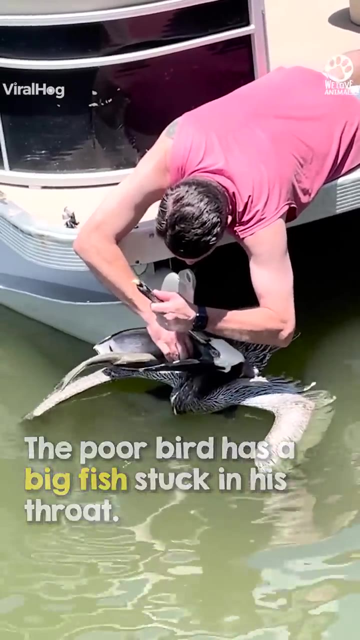 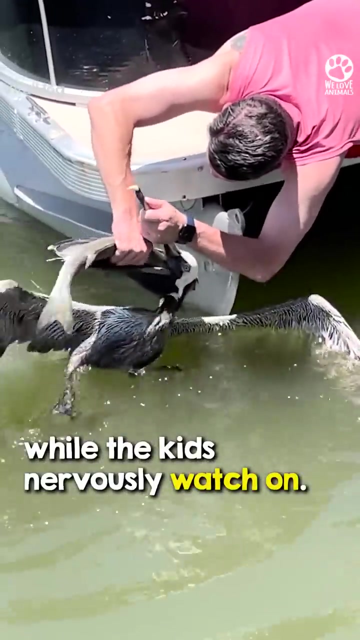 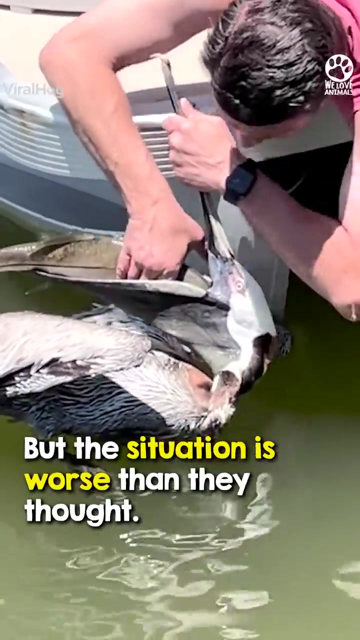 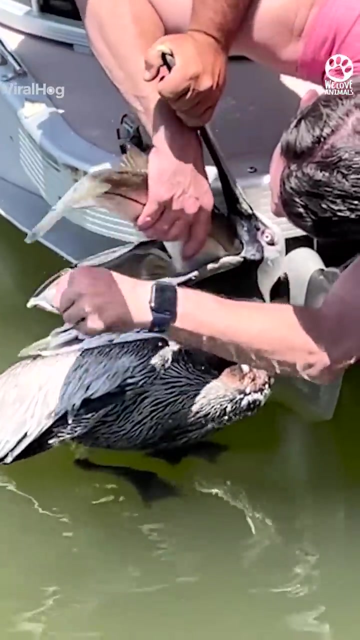 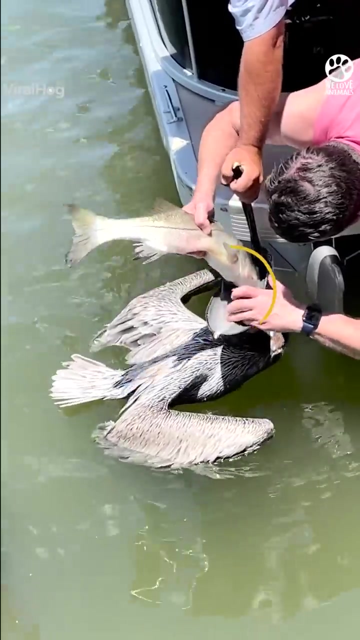 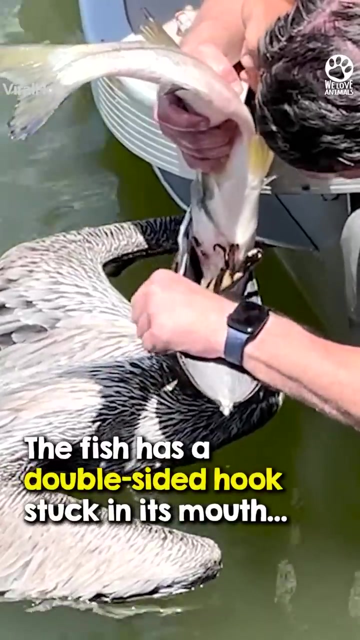 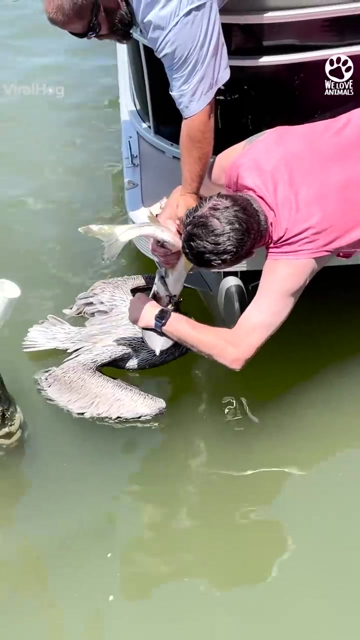 He's choking. Hurry, save him. Get it, Save him. He's trying to get him detached. He's choking. Oh, he's got a hook in him. Oh, he's got a hook in him. That's a bird call. We're saving the pelican.